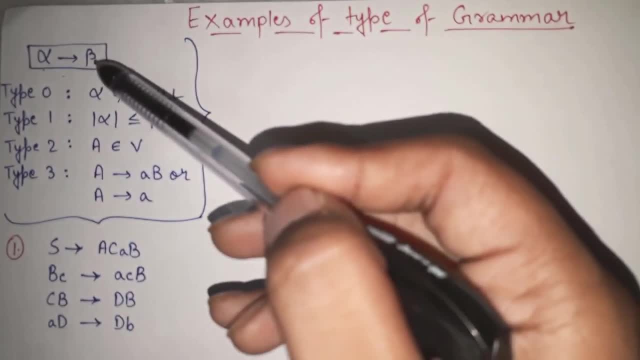 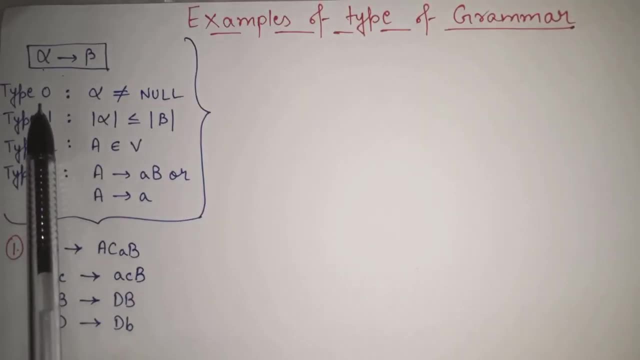 So see, as I told, alpha gives beta will be the general form of our grammar. Fine, Now If I want to see if this is type 0 grammar or not, then the thing or the condition that should not be violated is in type 0, the condition, the most important condition, is alpha must not be equal to null. 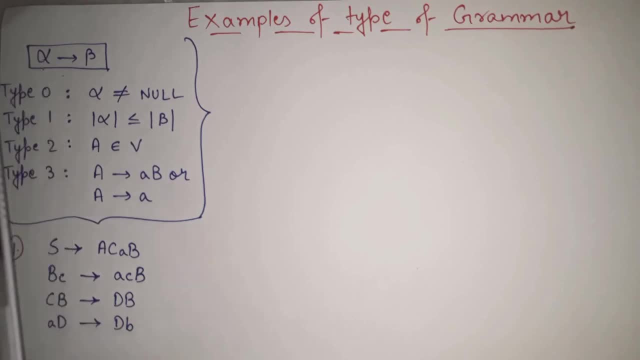 This alpha or the LHS must not be equal to null in type 0. This is the main condition. The main condition of type 1 grammar is the length of alpha. This modulus alpha means what Length of alpha? The length of alpha must always be less than or equal to the length of beta. 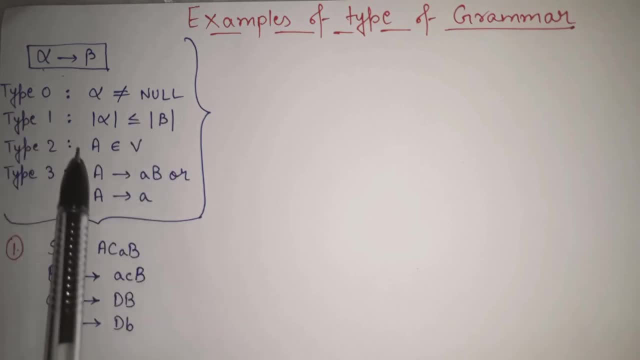 This is the main condition of type 1.. The main condition of type 2 is alpha. Okay, This is not a. Consider it as this alpha, This alpha must always belongs to one variable. That means what In type 0 and type 1, in this LHS or in alpha, both the combination of variables and terminals are possible. 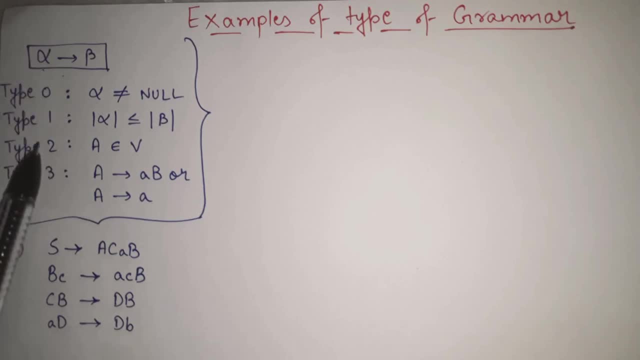 But if we talk about type 2. In type 2. LHS must consider only one variable. No other possibilities is there? Fine, So alpha part or the LHS part must always contain one and only one variable in case of type 2.. 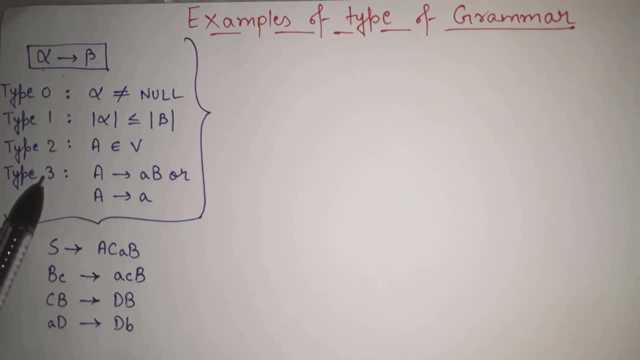 What is type 3?? The main condition of type 3 is: type 3 is what Regular grammar? That is the most restricted grammar. So in this, as this is the most restricted grammar, the main condition is: these are the only two variables. 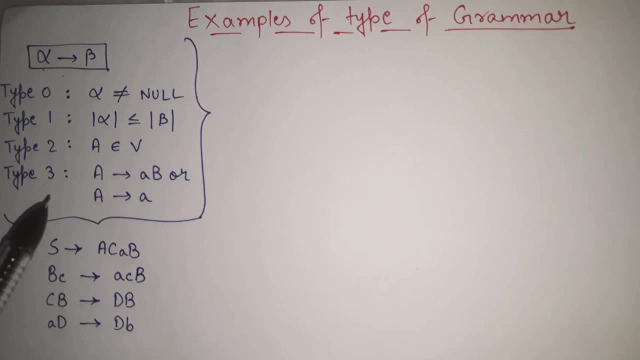 That is the only two types of grammar That is possible in this type 3. That is, allowing this type 3. Type 3 allows what A gives AB or A gives A. That means one variable giving. That means one variable giving only terminal or one variable giving the combination of terminal and variable. 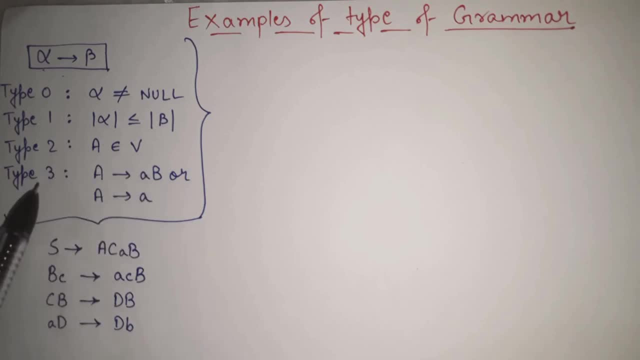 So this is the only possibility that is valid in case of type 3, regular. Type 2 is what? Context free language? Type 1 is context sensitive language. 0 is unrestricted grammar. so in unrestricted grammar, as the name itself indicates, it is. 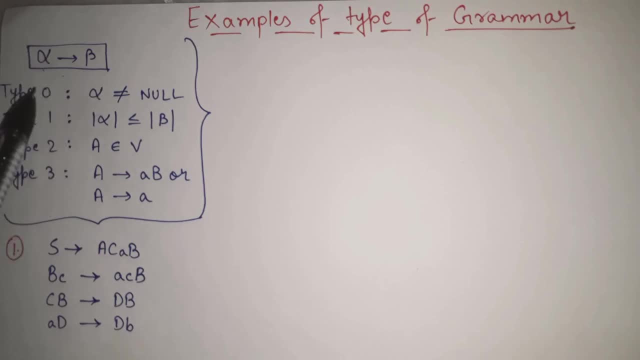 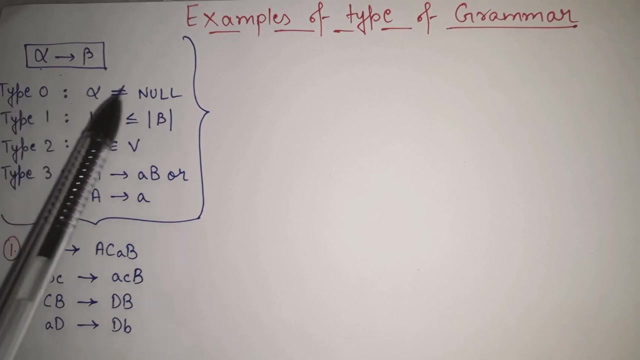 most unrestricted. that means in this there is no other restriction other than this, only one- that alpha is not equal to null and, as I have already in the previous video, I have shown you the relations also between these grammars. so, as per this relation, whatever condition is there in type 0, it will default be present in type 1, type 2, type 3, also in. 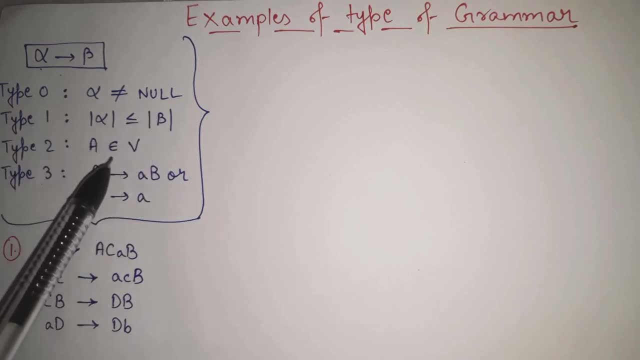 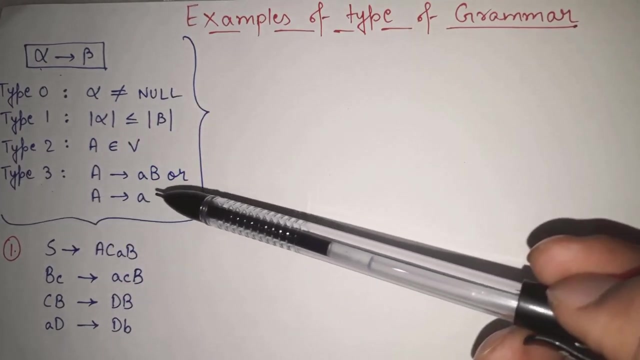 type 1. this restriction. it will be there in type 2 and type 3 also. this type 2 restriction will be present for type 3 also. so this is the relation between them. so type 0 is the most unrestricted, type 3 is the most restricted. this means what, if any of my grammar I can? 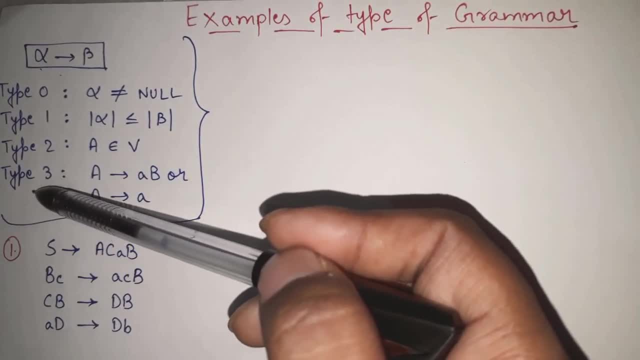 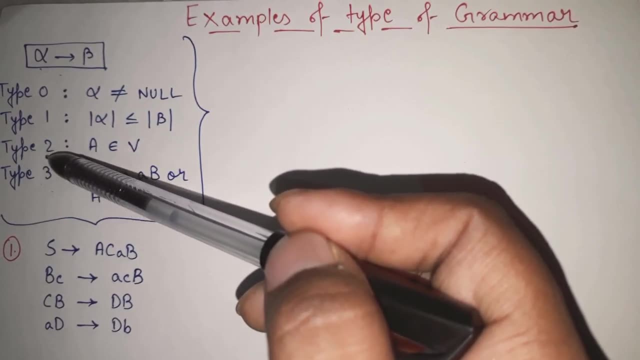 say, if any of the grammar is proved to be type 3, then I can say that it will be type 2, type 1 and type 0 also, If any grammar is type 2, then it will by default be type 0 and type 1 also. you are getting. 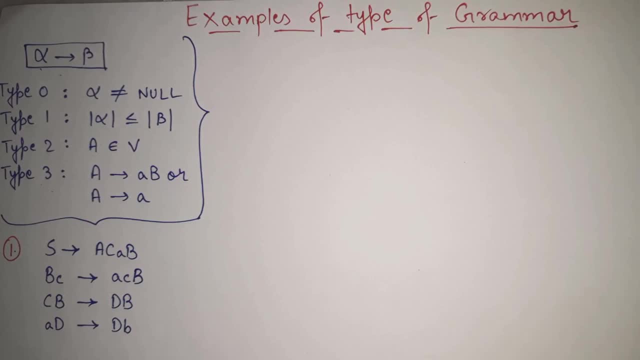 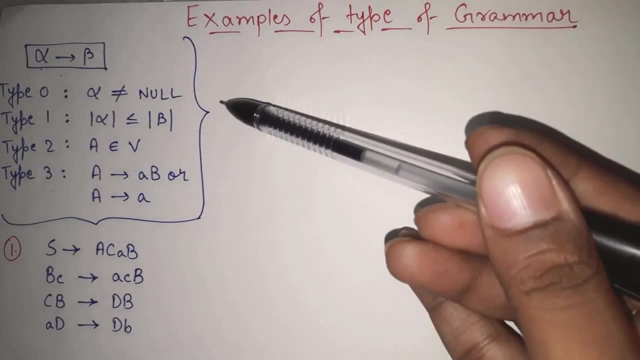 so the moral of the story is, whenever any grammar is given and we have to identify the type of the grammar, we will always start checking from the most restricted one. that means we will start checking from type 3 means if any of if type 3 condition is valid, I will simply. 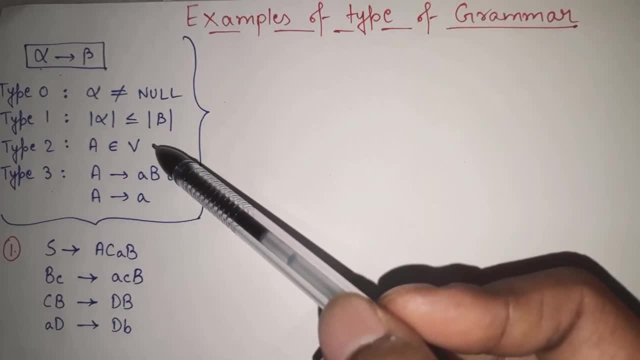 say that my grammar is type 3. if this is not valid, I will go to check type 2. if it is type 2, I can directly say that it is type 3.. Because it is understandable that if the grammar is type 2, it will by default be type. 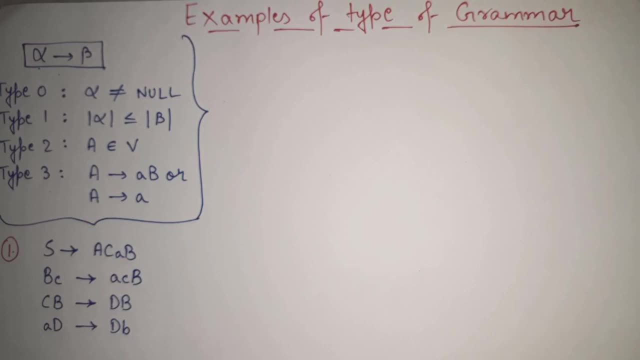 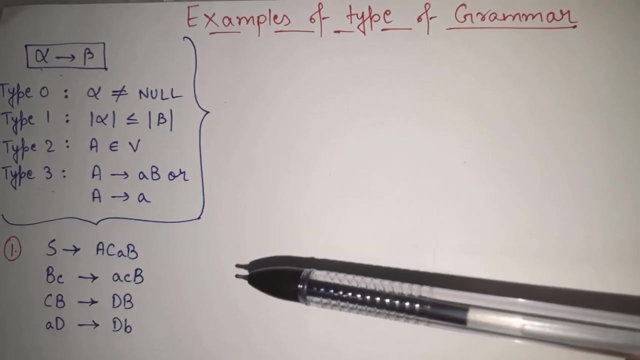 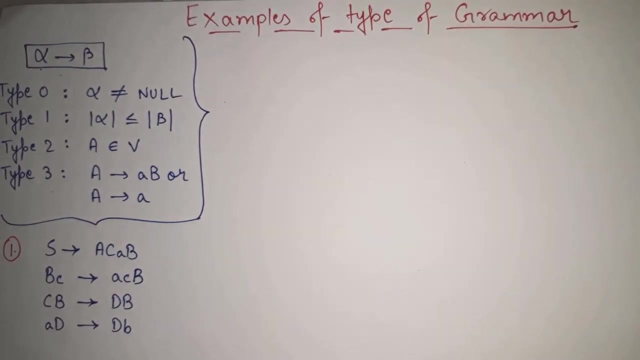 1 and type 0 also. so the things we have to keep in mind is these are the main conditions that we have to check, and we have to always check with the most restricted grammar, that is, we will always check from type 3, then type 2, then type 1, then type 0. these are the only. 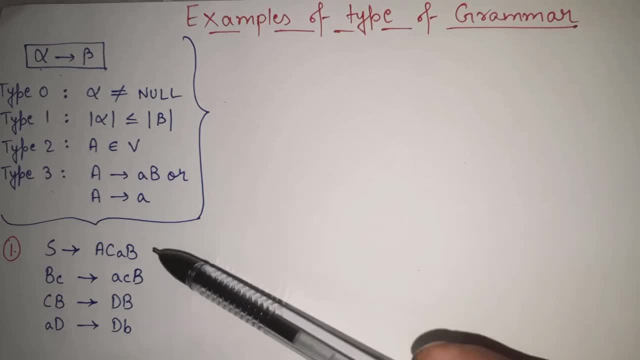 things that you have to keep in mind. ok, so let's see this first example. this is the first example of the grammar guide. So this is the first example of the grammar guide, and what we have to do is we have to just identify the type of grammar. so, as I told, we will start with type 3. what to check? 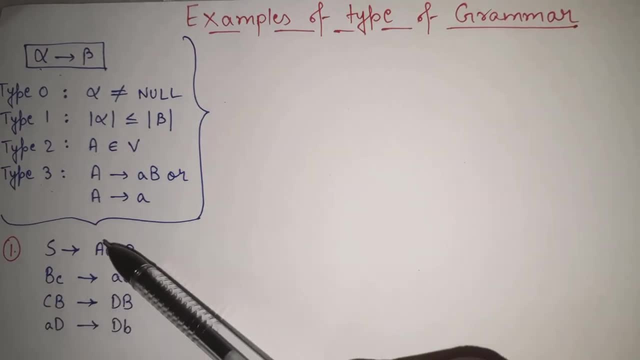 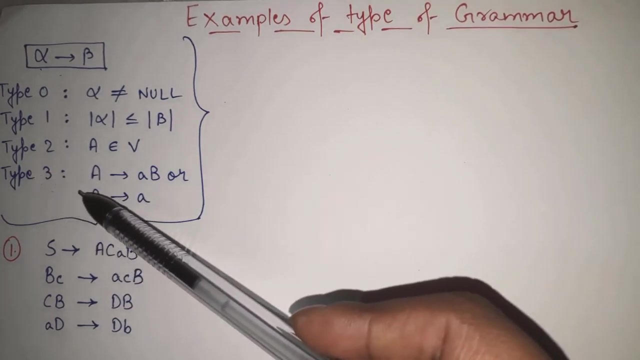 if this grammar is type 3 or not. what is type 3? saying that in LHS there must be only one variable and in RHS we can either have a terminal or we can have a combination of terminal and variable. so if we check, see, the simplest way to check is in type 3 and type 2, in both of 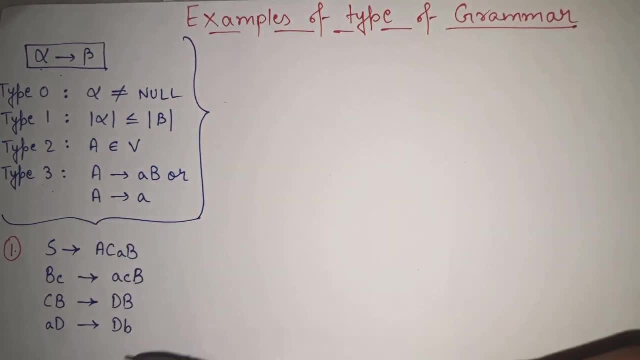 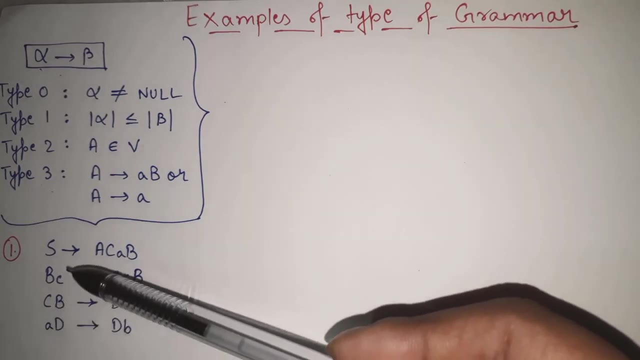 these types. So in LHS we can have only one variable, and you can see in the grammar that our grammar consists of variables and terminals both. so here also we are having variable, terminal, variable, variable, terminal, variable. what is variable, variable is nothing but non terminals. all the capital letters, capital letters, are variables or non terminals, and this small. 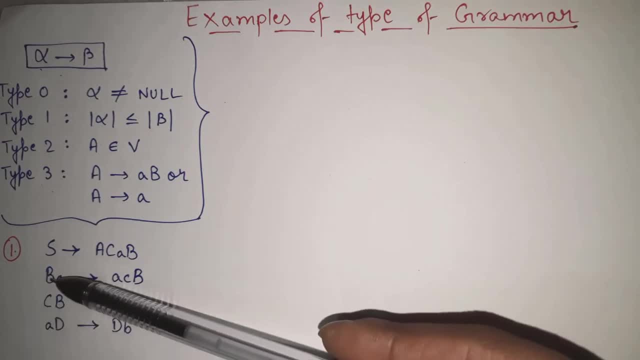 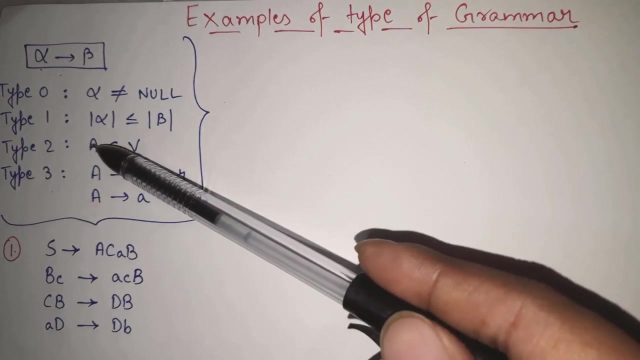 letter small c, small a, they are terminals. so we can clearly say: see this, that LHS is consisting of the Combination of terminals and non terminals. so we can directly come to the conclusion that it can neither be type 3 nor type 2, right, because in type 3 and type 2 we want only. 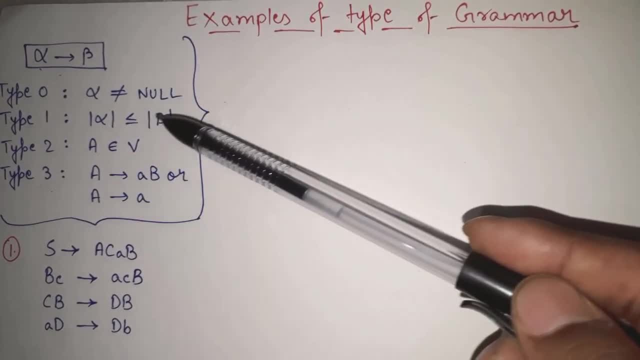 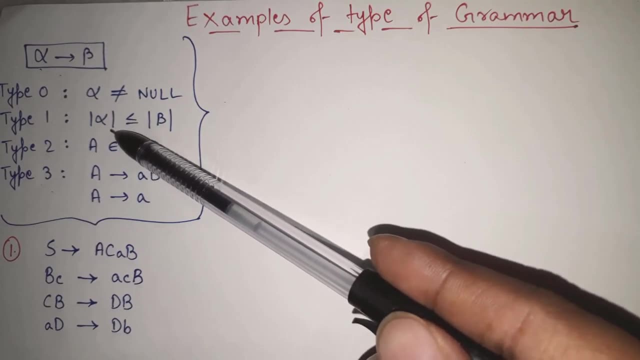 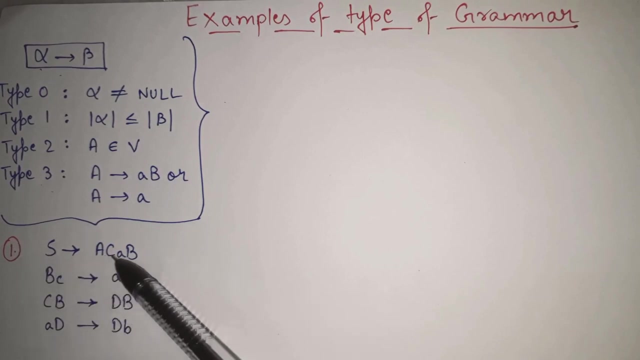 variable in the LHS. so next step is we will check for type 1. so what is type 1? the only condition that we have to check for type 1 is the length of alpha must be less than or equal to length of beta. so the length of this, the length of this is 1 and the length of 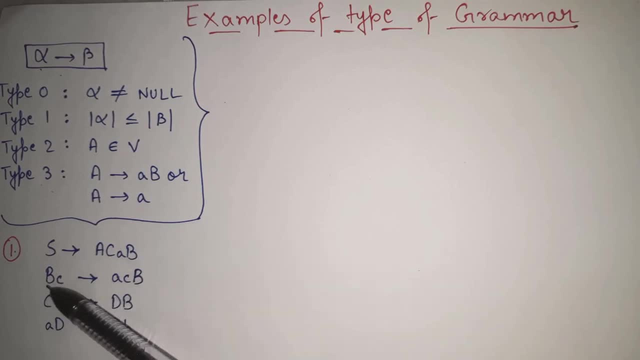 this is 4.. 1 is less than or equal to 4. right 2 is less than or equal to 3. correct 2 is less than or equal to 2. correct 2 is less than or equal to 2. this is also correct. so all the conditions. 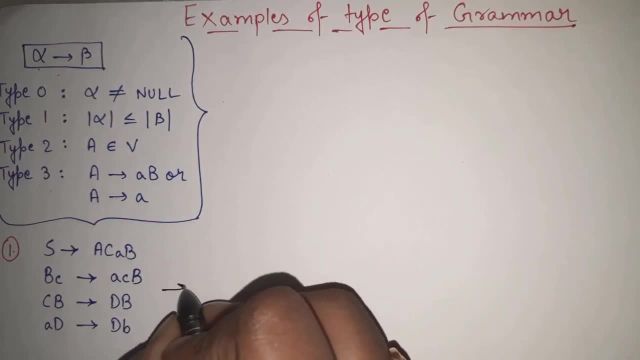 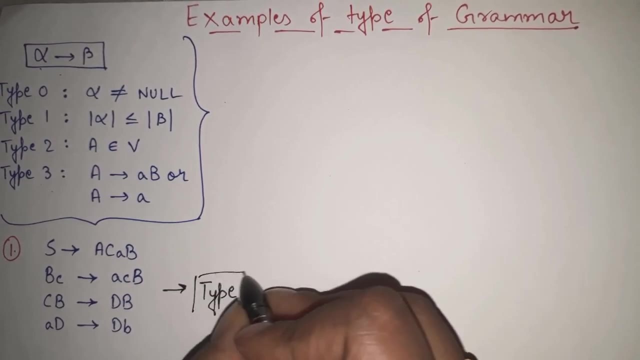 of type 1 are satisfied. so I can simply say that my this given grammar is under the category of type 1 grammar. type 1 means what context sensitive grammar, so I can say that this is my type 1 grammar or context sensitive grammar. Now, whenever I am saying type 1, it is understood that if it is type 1, it is obviously be type. 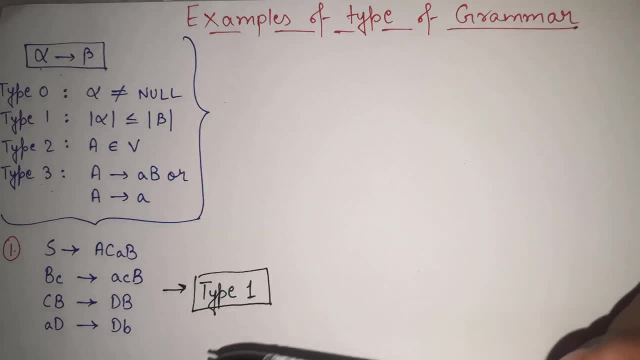 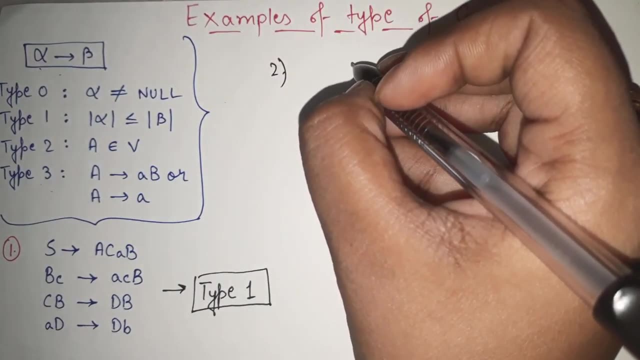 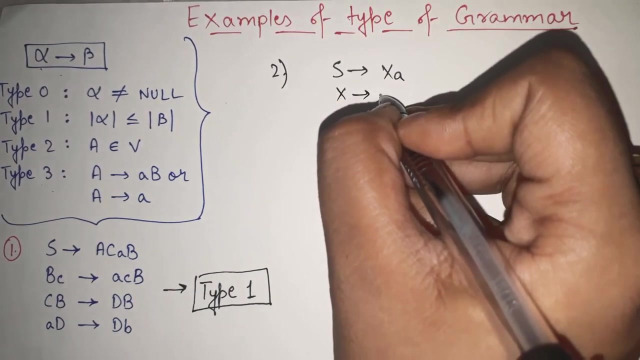 0 also. so my this grammar is type 1 and type 0, but not type 2 or type 3. fine, let's see another couple of examples quickly. for example, I am having S gives X A X gives small a X gives small a X. 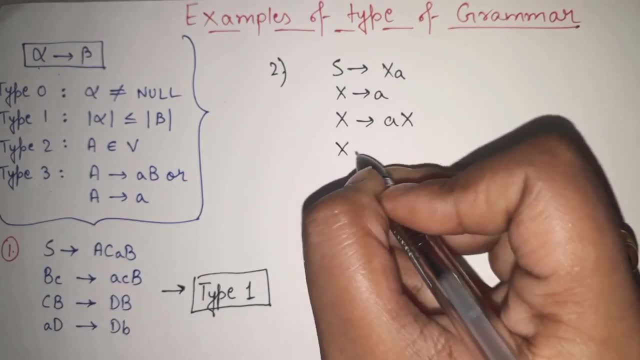 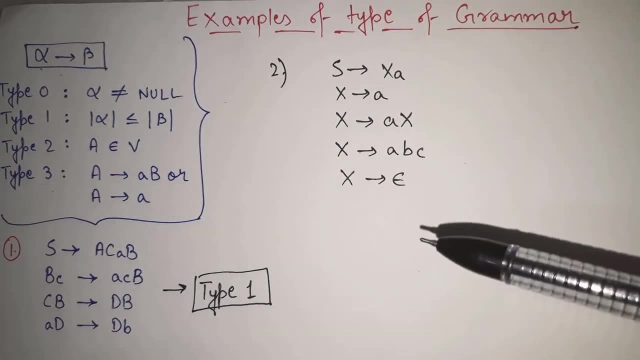 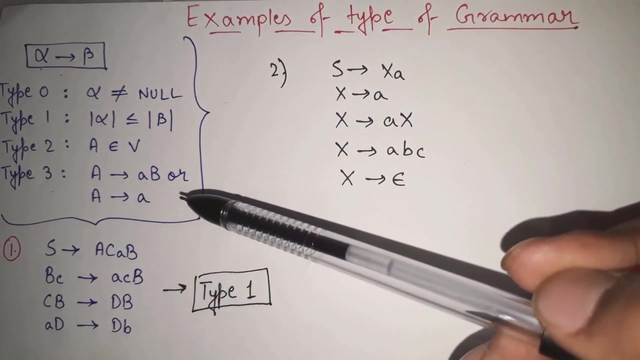 Then, Then, Then, Then, Then. X gives small a, small b, small c and X gives null. Now again, this is the grammar. I have to identify the type of grammar. I will start from the most restricted one, that is, I will start from checking type 3. again in type 3, my condition. 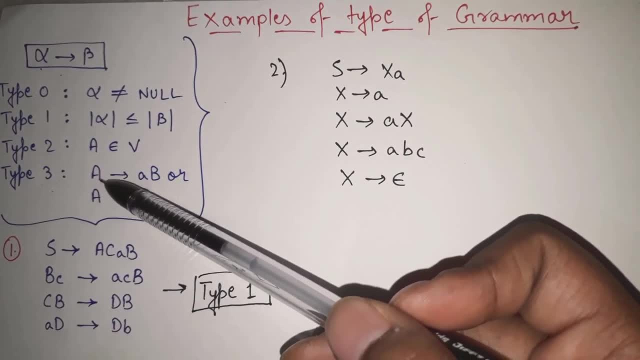 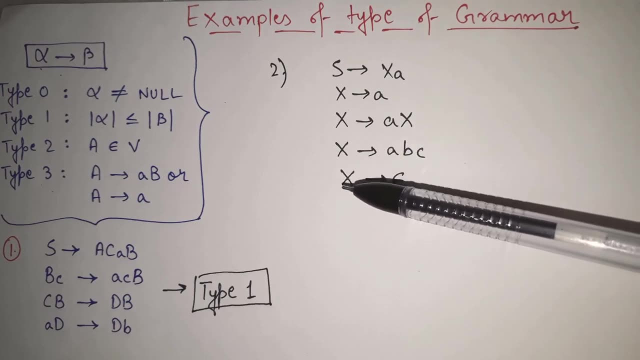 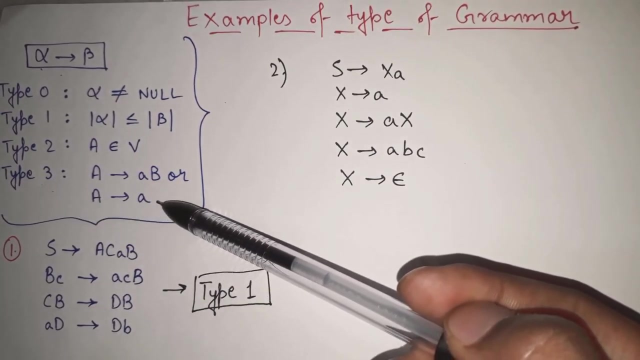 is first condition that I have to check is LHS must always be only one variable. so yes, all the LHS are only one variable or non terminal. that means my this condition is satisfied. fine, Now the RHS. in type 3, the RHS can be only terminal or the combination of terminal and. 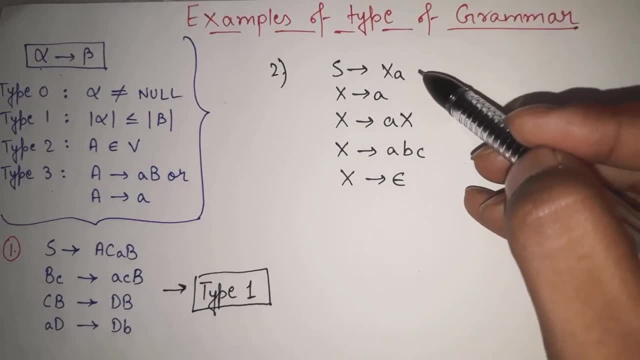 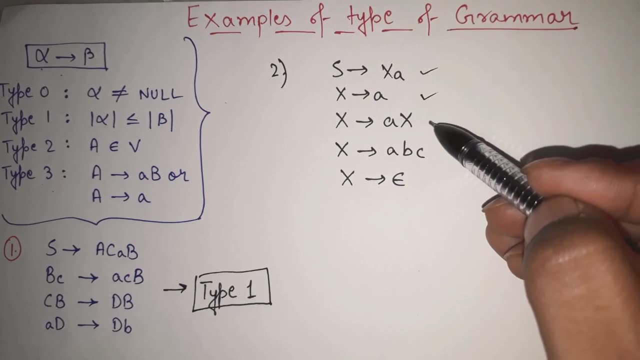 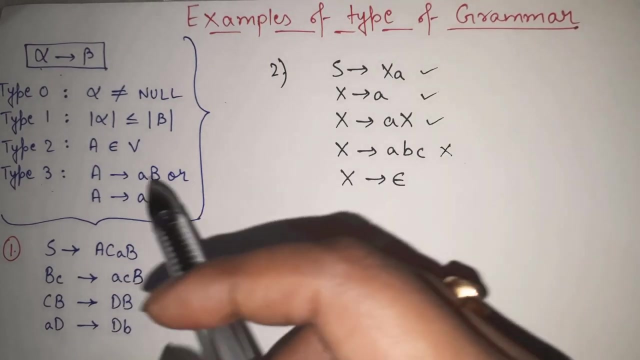 variable. So let me check here: this is terminal one terminal, one variable, correct. this is only terminal, correct. one terminal, one variable, correct. but no, here I am having three terminals and this is not satisfied in case of type 3.. So I can simply say that my this grammar is not type 3.. 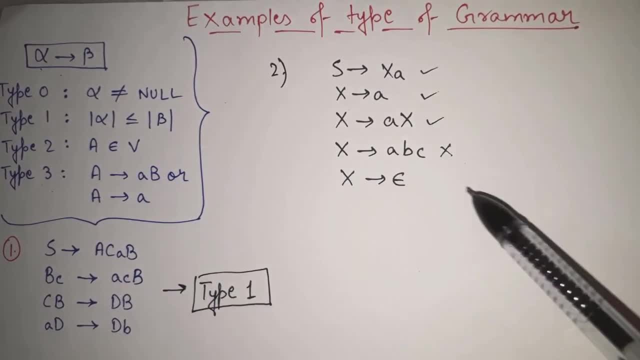 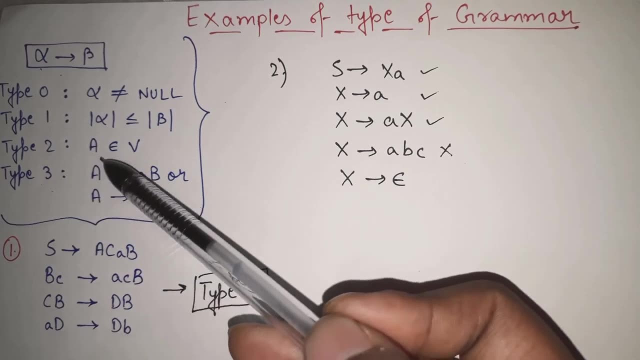 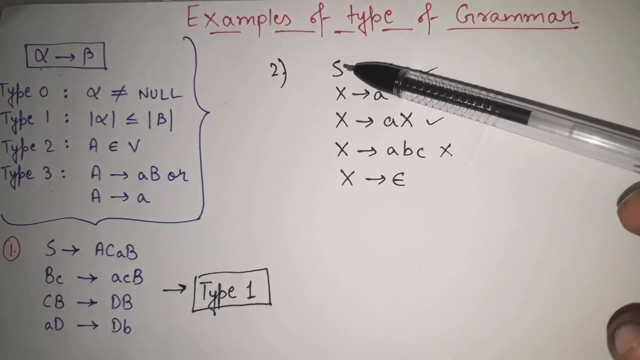 Got getting. this is violating the type 3 condition, So this cannot be type 3.. So we will go to check either it is type 2 or not. In type 2 the only condition I am having is that alpha, that is LHS, must belong to variable. that means LHS should be only variable or one variable. So yes, 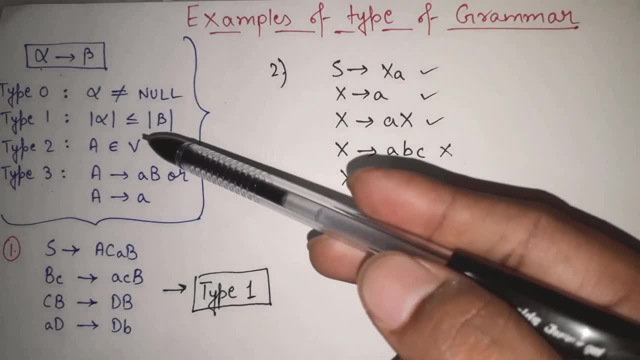 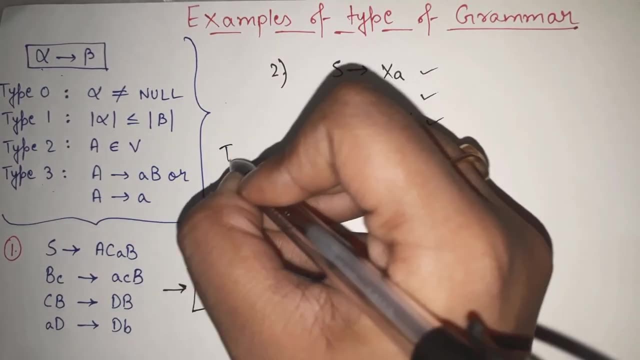 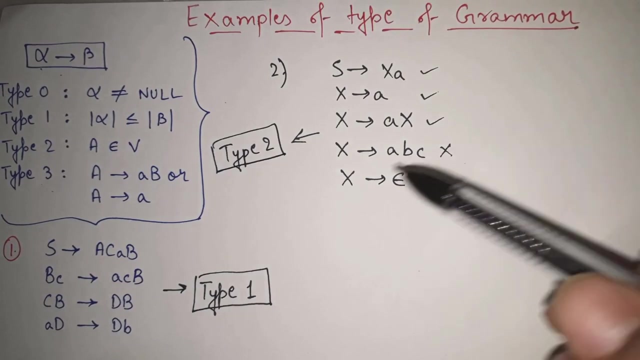 all the LHS here is just a variable and no other critical condition is there in type 2.. So simply I can say that, yes, my this grammar is type 2 grammar. What is type 2 grammar? Context tree grammar. Type 2 grammar is context tree. I can say that my this grammar is type 2. 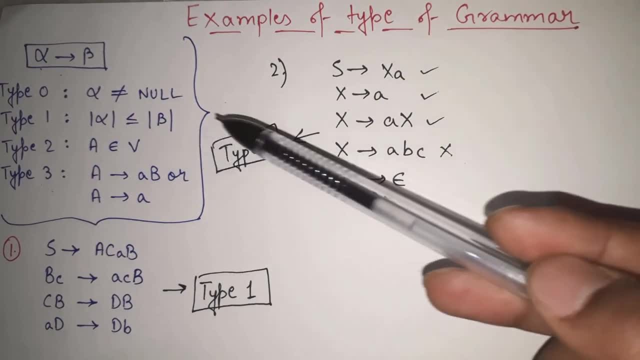 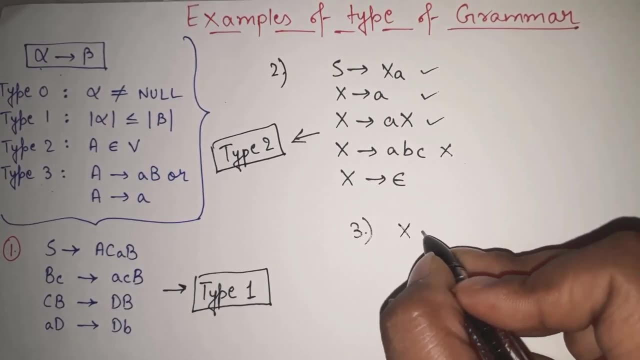 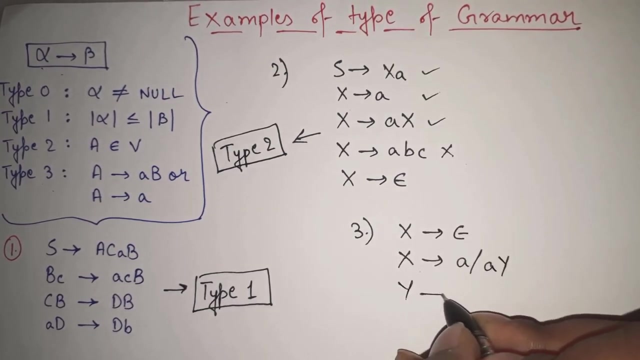 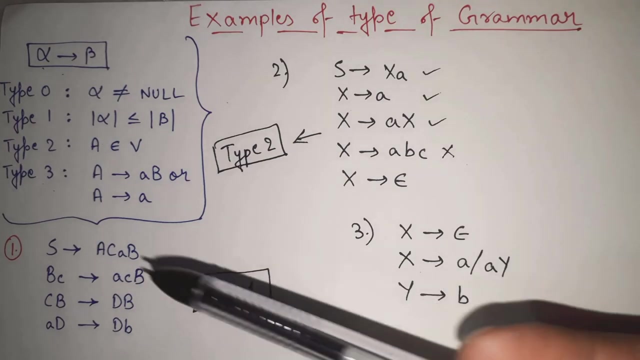 or context tree grammar. Now, as I told, as it is type 2, it is automatically type 1 and type 0 also. Fine. Let's see another example: X gives null, X gives A or AY and Y gives B. Fine, So this is my given grammar. We have to check that which is the type of grammar. We will start with type 3.. 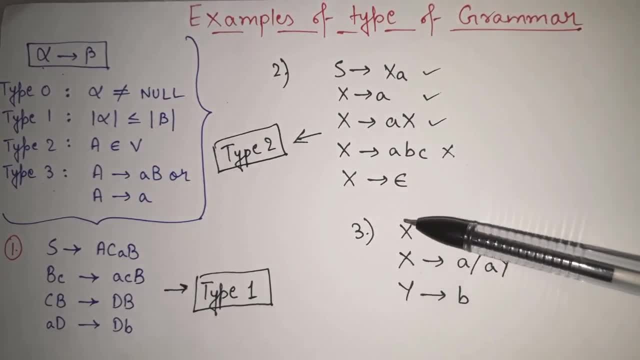 In type 3. all the LHS must be variable. Yes, all the LHS are variable. RHS must contain only terminal or the combination of terminals and variables. This is only terminal, Only terminal or terminal and variable. yes and X gives null is also valid, unless this X is present in any other RHS also. 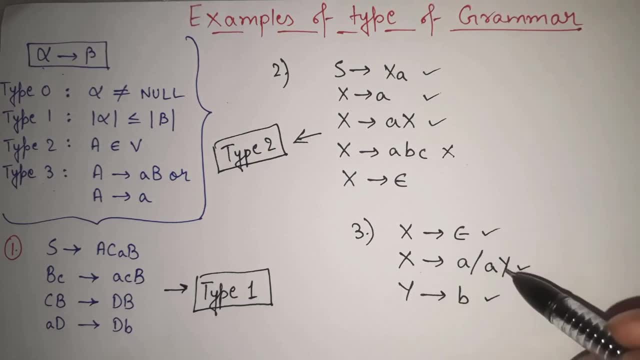 So, yes, this is also valid. So in this case, all the productions are satisfying the type 3 conditions, So I can say that I don't need to check further. I can simply say that my this grammar is type 3.. Type 3 means what? Regular grammar? So I can say that my this grammar is type 3 or regular grammar. 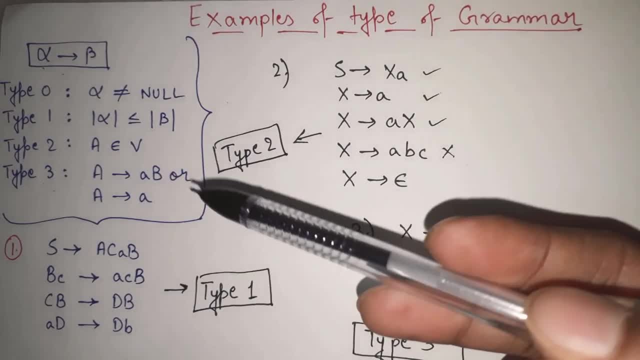 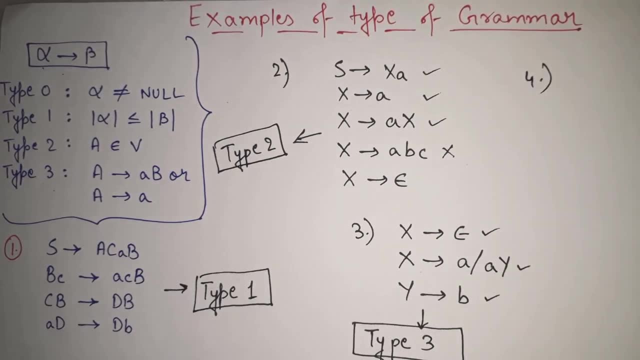 And, as I told, as it is type 3, it will automatically be type 2, type 1 and type 0 also. So let us take one more example. As you will practice more and more example, you will get a more clear idea, right. 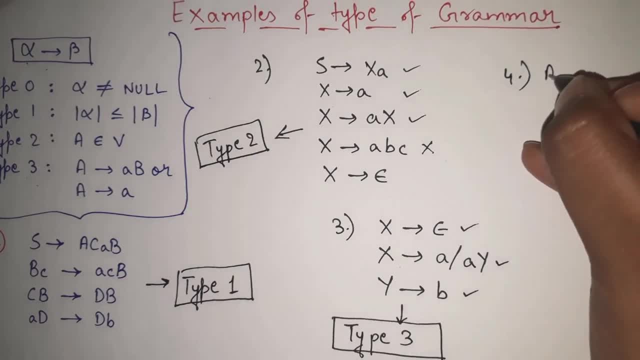 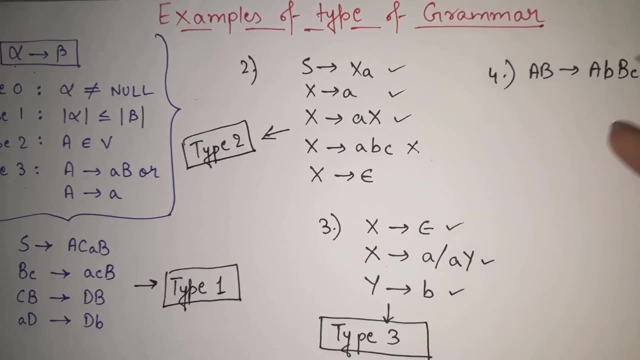 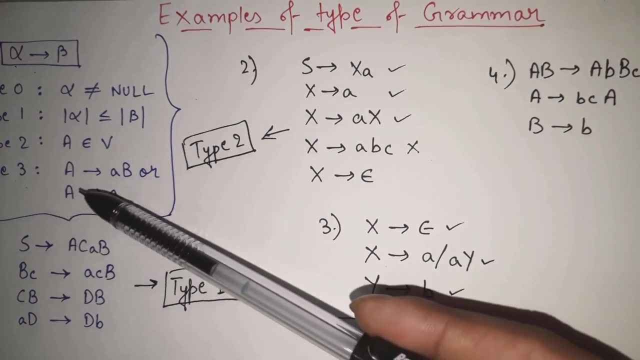 So let us see one more example: AB gives AB BC, AB gives AB BC, then A gives BCA and B gives B. So first of all, if I check about type 3.. In type 3 again in type 2 and type 3, both the LHS should contain only one variable. 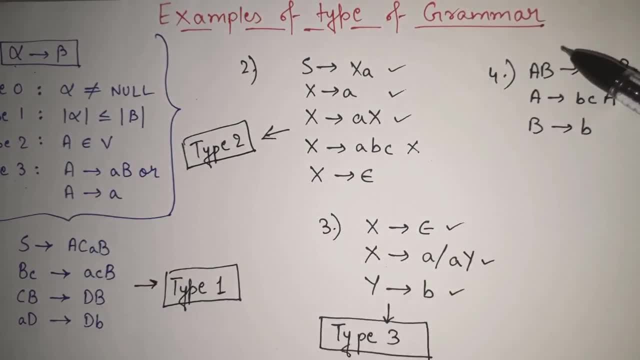 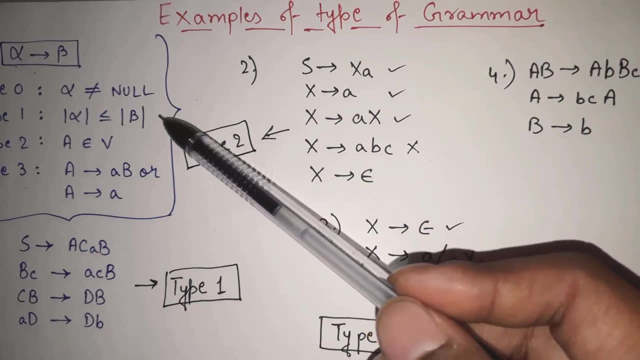 But here, if I check the, here, the LHS is containing more than one variable. So it is clearly seen that it cannot be type 3 or type 2.. So the next thing is you will go to check for type 1.. In type 1, only condition is the length of alpha is less than or equal to length of beta. 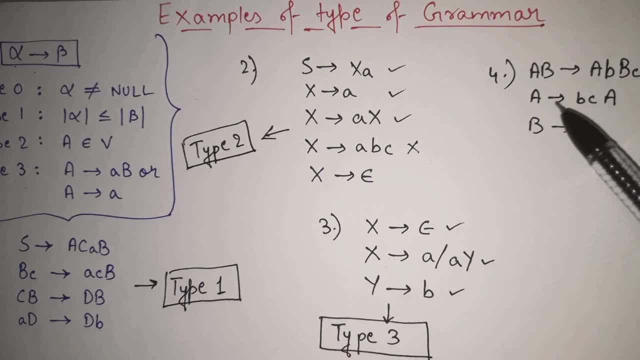 So 2 is less than or equal to 4.. Yes, 1 is less than or equal to 3. yes, 1 is less than or equal to 3. yes, Vamos a verificar. второй conditioner remaining is less than or equal to 1,. yes, so it is satisfying all the conditions of type 1, so. 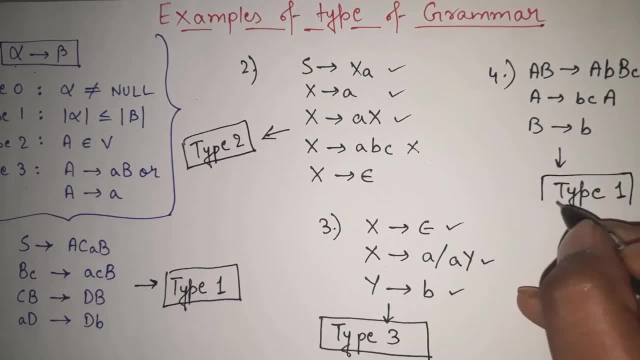 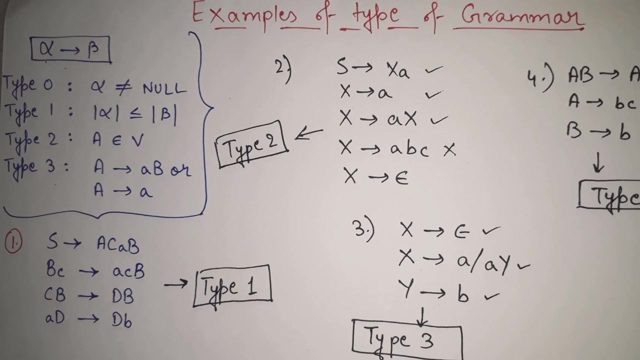 my this grammar is type 1, type 1 means what context sensitive grammar and again, as it is type 1, it will be type 0 also fine. so these are some of the examples that to know that how we can check the type of grammar correctly and very easily and quickly, I hope. 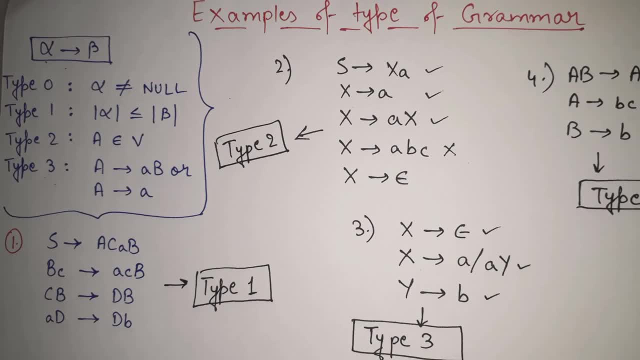 you have understood it. in case you still have any doubt, you can always ask in the comment section. thank you so much.